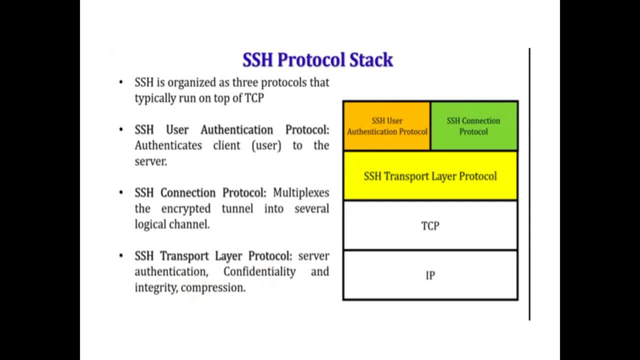 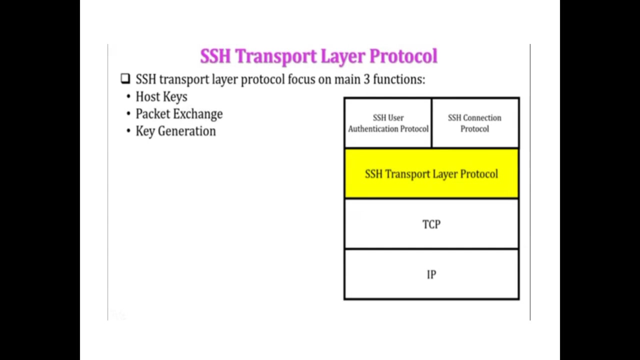 SSH connection protocol. multiplex: the encrypt tunnel into several logical channel. SSH transport layer protocol. server authentication, confidentality and integrity compression. and this is the diagram of SSH protocol stack. SSH stands for layer protocol. focus on the C main functions there are Host key, packet exchange, key generation. and this is the diagram of SSH transport layer. 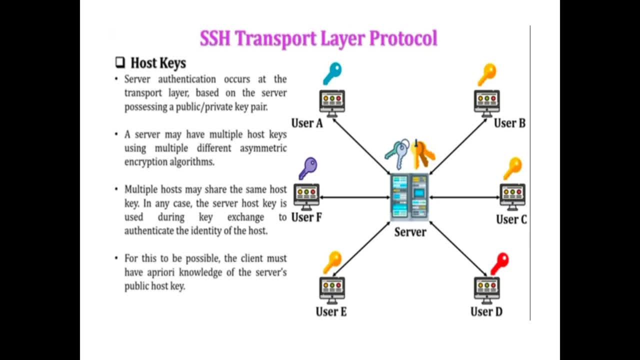 protocol. transport layer. protocol consists of Host key. this is the diagram of Host key here: server user: a user be user see user D. user F, user E: user F: server authentication occurs at the transport layer based on the server processing a public-private key pair. a server may. 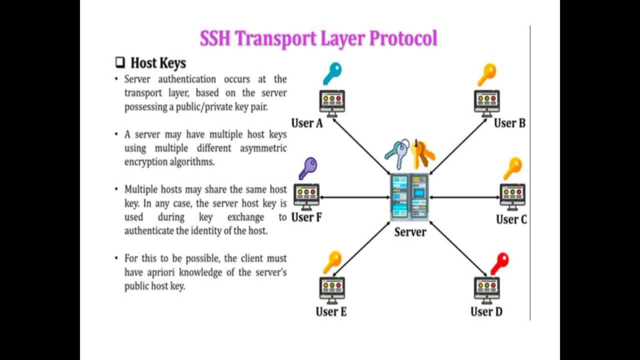 have multiple host keys. using multiple different asymmetric encryption algorithms, multiple host key may share the same host key. in any case, the server host key is used during key exchange to authenticate the identity of the host. for this to possible, the client must have prior knowledge of the server. 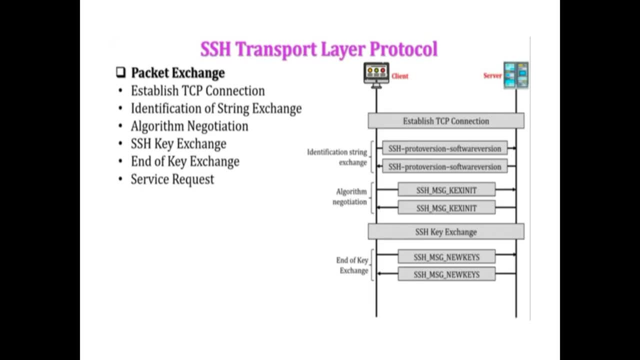 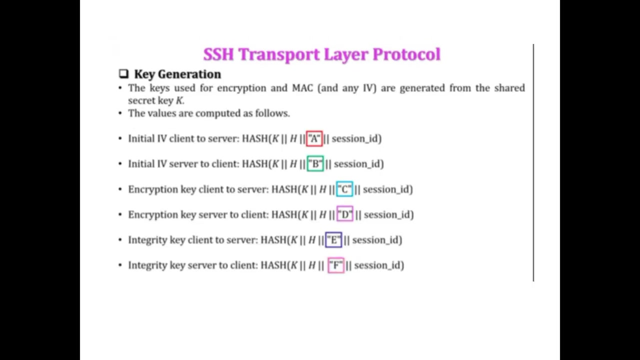 public host key. SSH transport layer consists packet exchange. here this is the diagram of SSH transport layer protocol packet exchange client server and it consists of: established TCP connection, an identification of string exchange algorithm navigation. SSH key exchange. end of key exchange server request key generation: the key user for encryption and emacy are generated for the she and 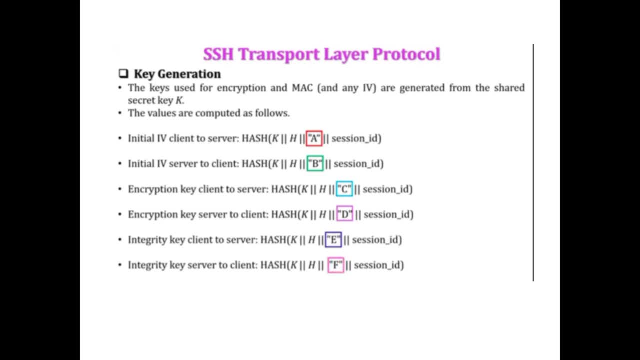 secrets- key K. the values are computed as follows: initial fourth subcommittee client to server hash: kha session id. initial fourth server to client hash: khb server id encryption. key client to server hash: khc session id encryption. key server to client hash: khd server id integration. key client to server hash: khe server id integrity. key server to client hash. 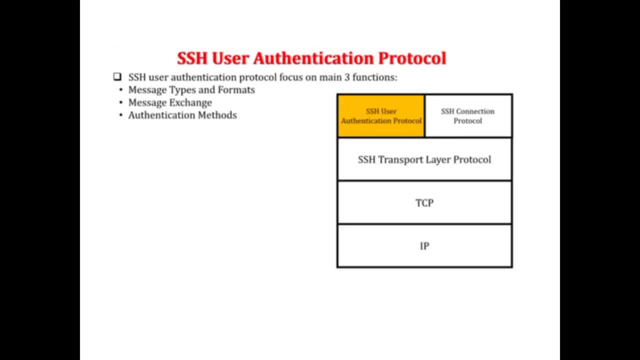 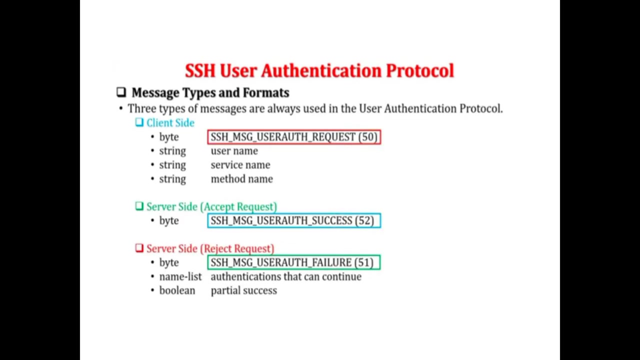 khf session id. now let us see the user authentication of ssh. ssh user authentication protocol focused on three main functions. there are message types and formats, message exchange, authentication methods. here, message types and formats, three types of messages are always used in the user authentication protocols. there are client side, server side, accept request and the last one is server side. 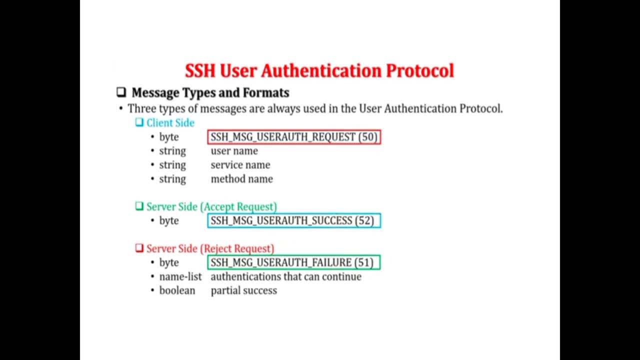 reject request. client said: byte ssh message: user authentication request: 50. string username, string service name, string method name: server said: accept request: byte ssh message: user authentication success: 52. server side: reject request: byte ssh message: user authentication failure: 51. name list authentication. that can continue: boolean partial access ssh. 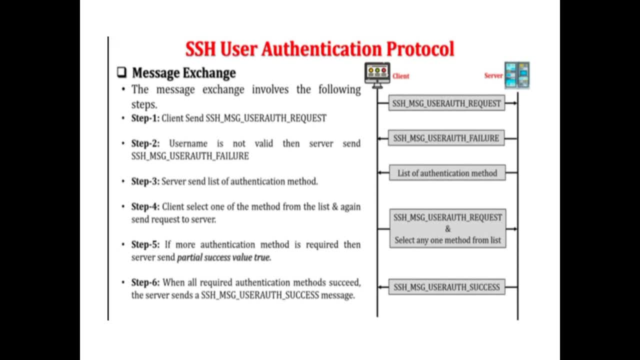 user authentication protocol in message exchange. the message exchange involves the following steps. it has six steps. in the first step, client send ssh message- user authentication request. and in second step, user name is not valid, then server and as such measure user authentication failure. step 3: server sends list of authentication method. 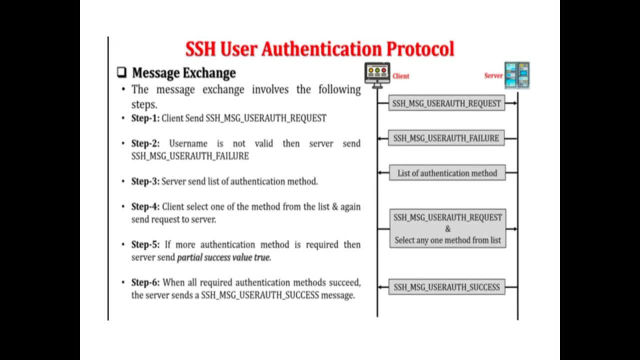 fourth step: client select own one of the method from the list and again send it to the server. fifth step: if more authentication method is required, then server send partial success value: true. and the last step, 61, when all required authentication methods success. the server senses ssh message. user authentication success message. 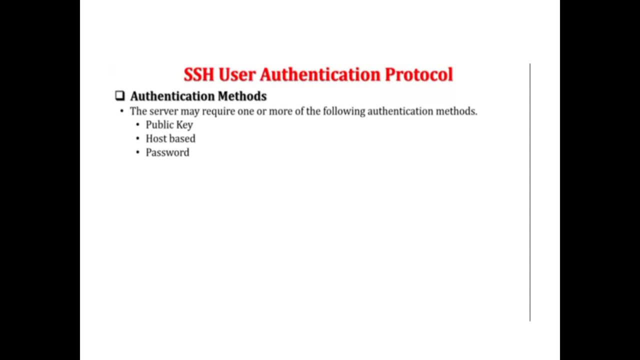 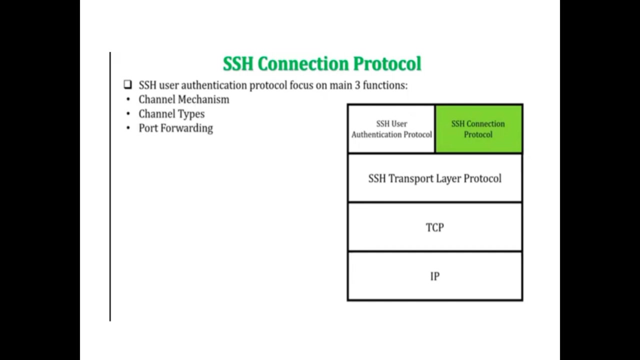 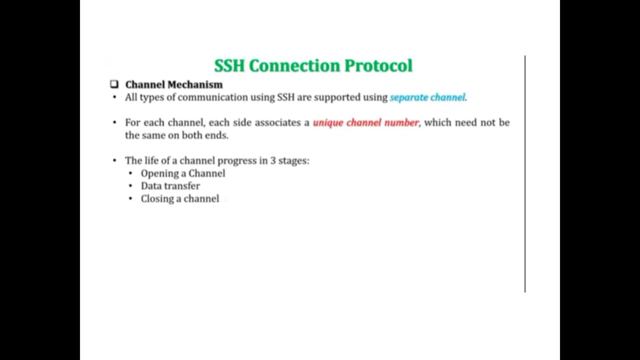 next at an authentication methods. the server may require one or more the following authentication methods: from ssh source about the server. data from the permission of the server or from the detected server policies important for authenticationData. port pass vehicle. all the types of communication using SSH and supported using separate channel for. 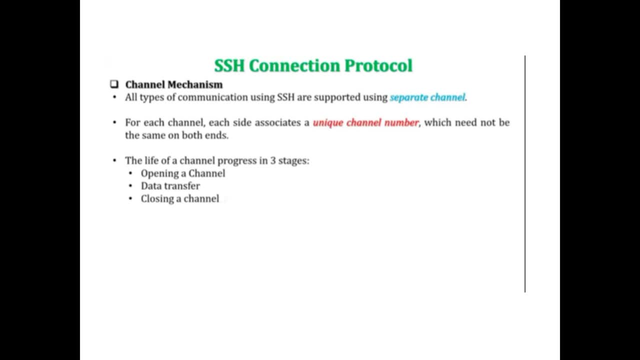 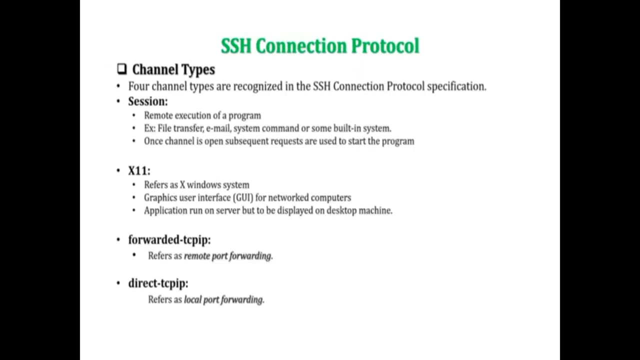 a channel, each side as associates a unique channel number, which mean not to be the same, and both ends life of the channel progress in three stages. there are opening a channel, data transfer, closing a channel and channel types, for channel types are recognized in SSH connection protocol specification. 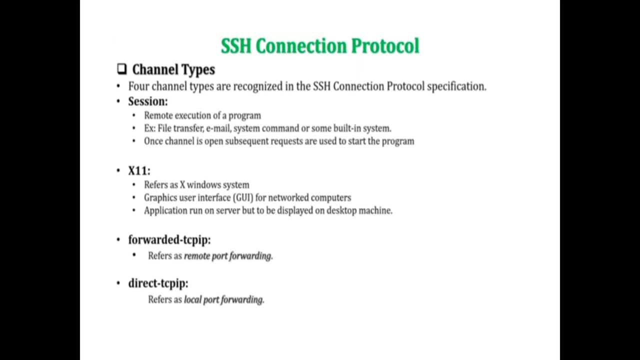 session remote execution of a program, example file transfer, email system command or some built-in system. once channel is open, subsequent requests are used to start the program. X level refers as X window system graphics user interface for network computers. application unknown server but to be displayed on desktop machine. 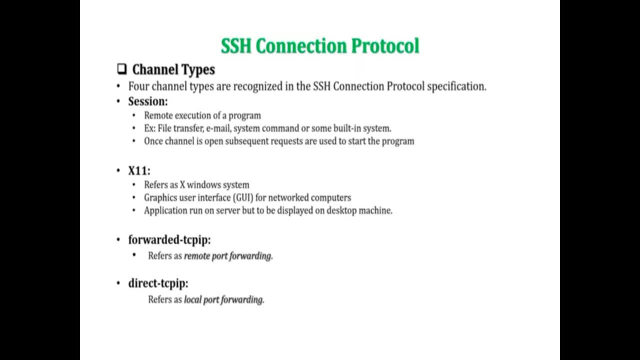 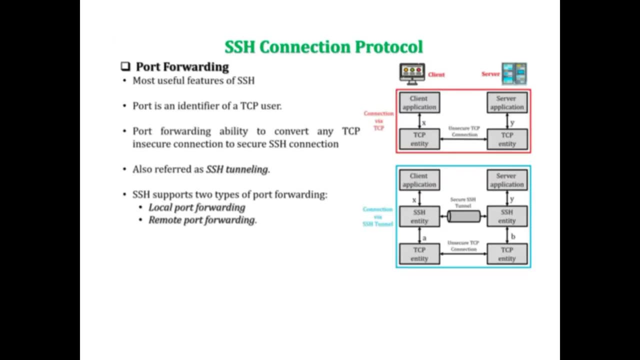 forwarded TCP IP refers as remote port forwarding. direct TCP IP refers as local port forwarding. port forwarding most useful features of SSH port is identifier of TCP user. port forwarding availability to convert any TCP in secure connection to secure SSH connection also refers as SSH tunally. SSH supports two types of port forwarding. there are: 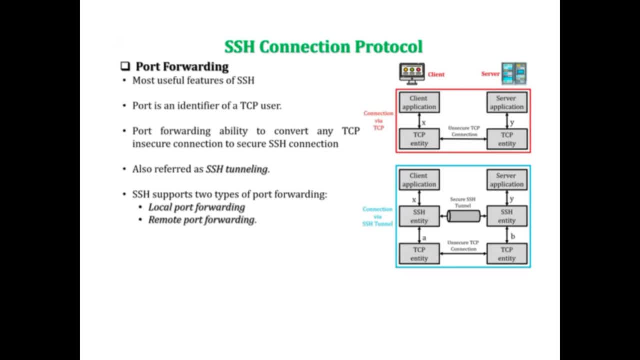 local port forwarding and remote port forwarding. connection protocol with it means to responsible to create tunnel into several logical channels and this is the diagram of connection protocol of port forwarding. thank you.